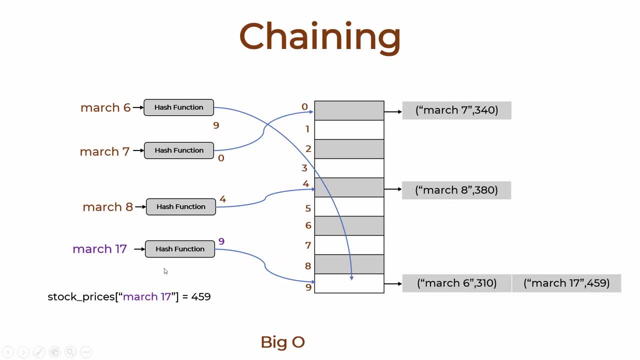 of a linked list which is order of n And when. now I want to retrieve the value of March 17,. first I use hash function to get an index which is nine. I go to index number nine. I linearly search this linked list And for that reason it is important to have your key stored. 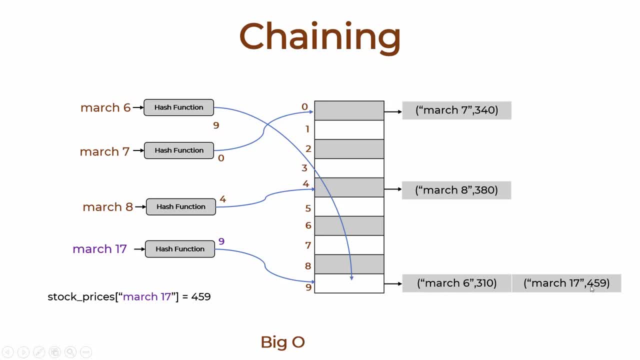 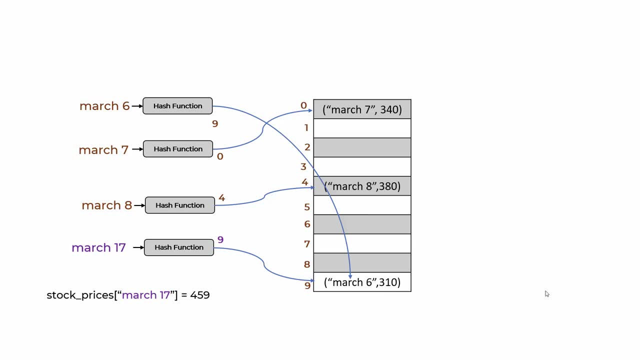 in each of these elements so that you know which value is associated with which key. The second approach for solving the collision is called linear probing. Here what we do is when, for March 17,. we get an index nine and we find that there is already a value stored at this location. 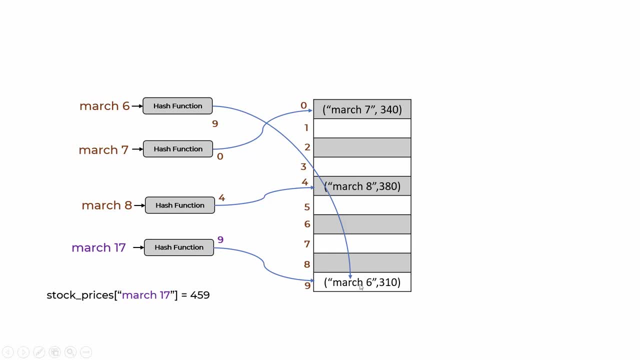 we go to the next available location Here. my array is ending here. But let's say, if there was a 10th location which was empty, then I would store March 17 at 10th location. But since I don't have 10th location, I will go reverse. look at 0th location. 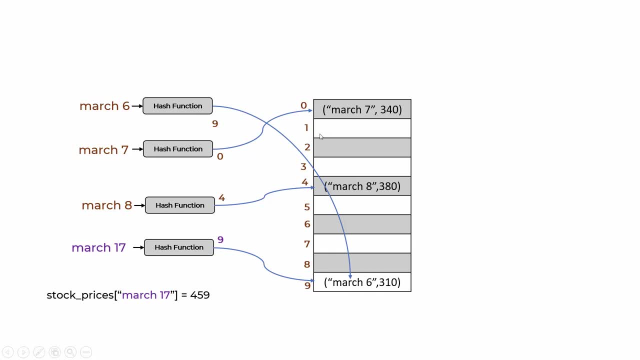 that location is also filled out. So then I go to location number one And here I store my March 17 value. It is called linear probing because I am linearly probing means search in for an empty slot to store my key value pair. I have another example where March 18. 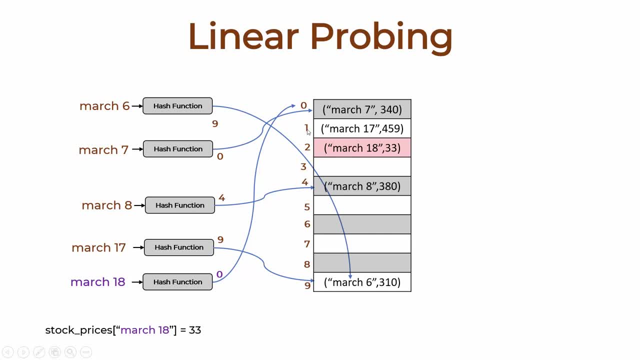 resolved to index zero. there was already a value, So we went to index number one. that is also filled, So now you store your value at index number two. Now let's implement chaining in Python. Here I have a Python class that we implemented in part one of this tutorial And 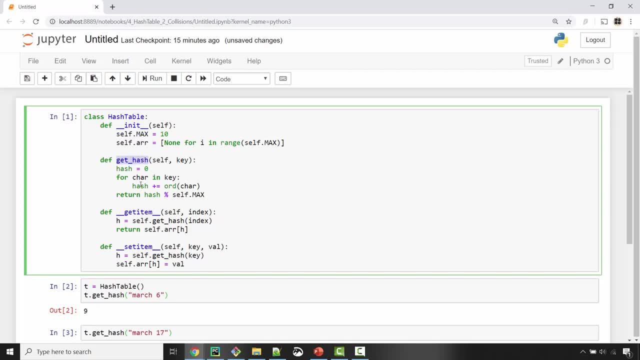 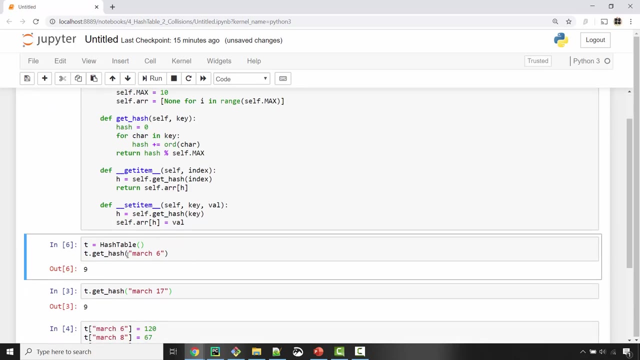 this class is not handling collision. All it is doing is getting a hashing function. And when you get a hash function it will go to a particular index in your array and store the value. I will show you what problem this class will have. So here I have a get hash function being called. 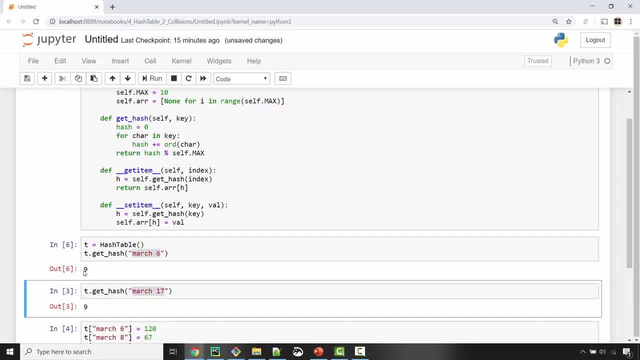 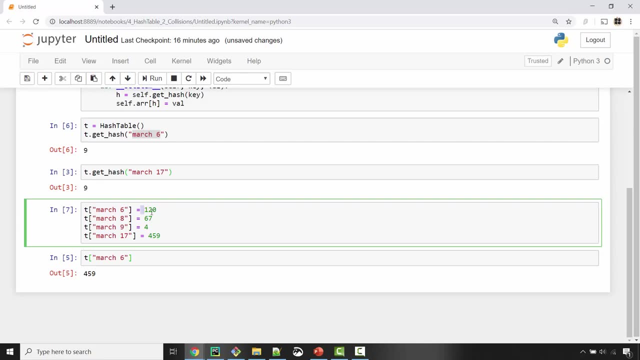 for March 6 and March 17.. And you know that they both have the same index. So when I store values like this for March 6, I have value 120, March 17, it is 459.. But since March 17 has the same, 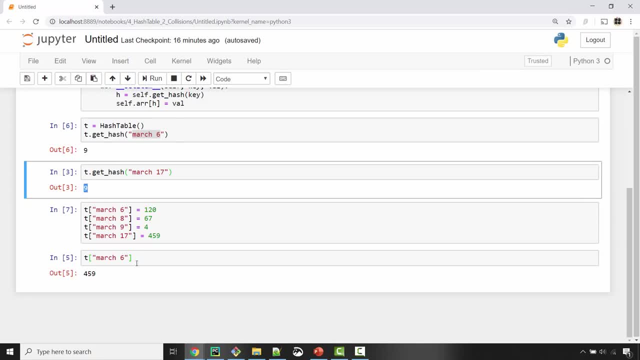 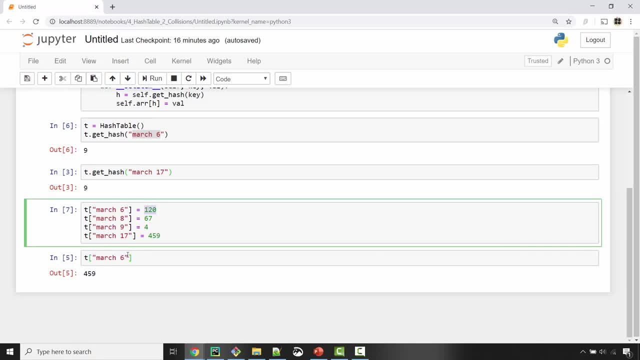 I am getting 459.. See, I stored 120, but I am getting 459.. And that is because of collision, because March 17, this 459 value overwrote that. So now we are going to fix that collision in. 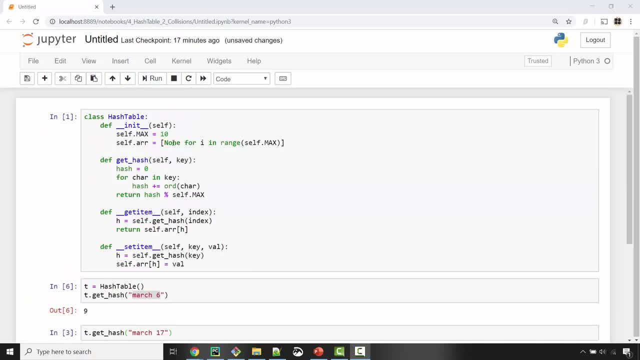 this same class. here, The first thing I am going to do is, instead of initializing none as individual element, I will initialize empty array, Because now each element is not just the value. we are storing key value pair. So, if you remember from our first presentation, we store key value pair whenever we have collision. 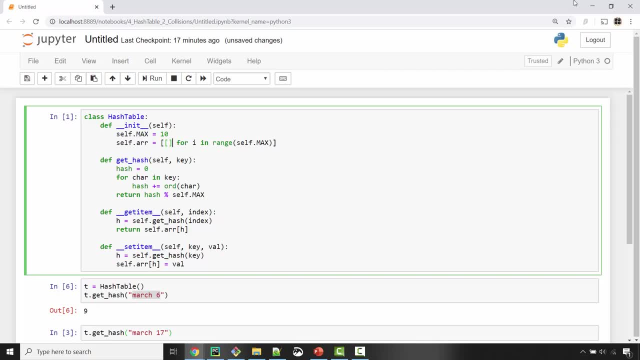 so that we can locate the right element. That's why I am having array in each individual element. The get hash function remains the same. We don't need to change that. We are now going to implement set item function. In our original implementation we used to. 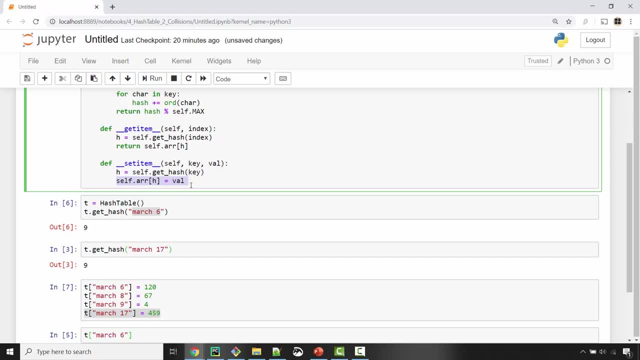 overwrite the value at index H. But at index H now we have a link list, So we need to iterate through the link list and find the right location to update our value. So the first thing we will do is in our link list if this element already exists. so it could happen that you might already. 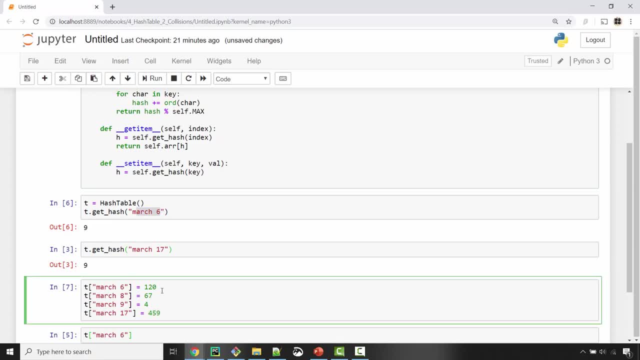 have as click box link list in your location and you will be like March 6,, let's update the value with something else, Freeze, And then in the end, if they come into the server, we skip that, So we can delete that and they will not see any link list. Still, let's keep generating changes. So. 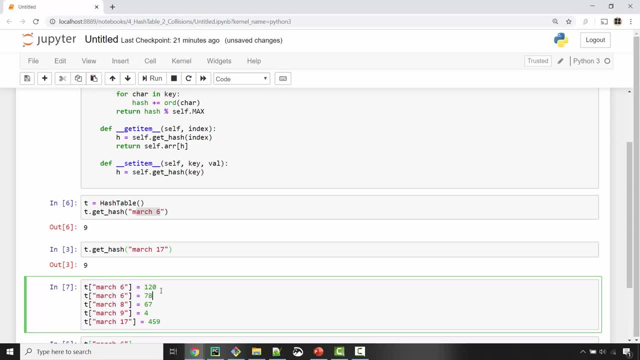 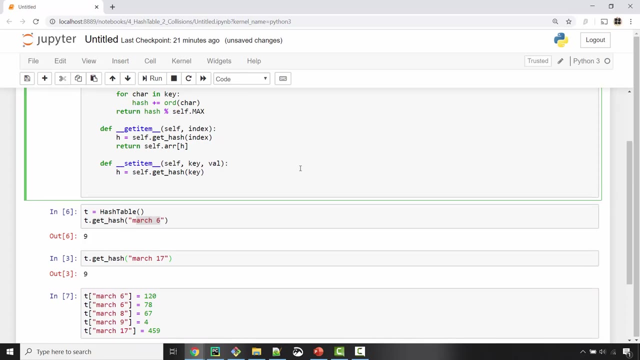 For example, here, if you have something like this, where initially you insert a mass six but then next time you want to update the same value, OK for that key. So we are going to handle this particular case first. So let's iterate through it Now. before we iterate through it, let me show you a simple case. 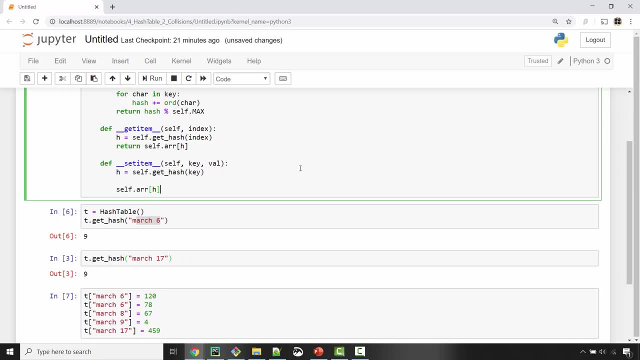 So let's assume that at this index or this particular key does not exist. In that case, what you will do is simply in that link list. So this, this particular thing, this one is a link list, or in Python, we are just using a list here. 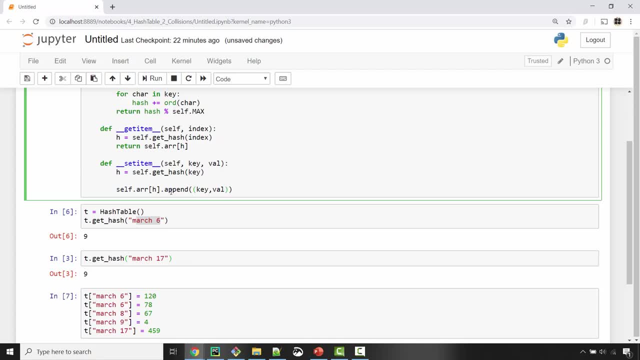 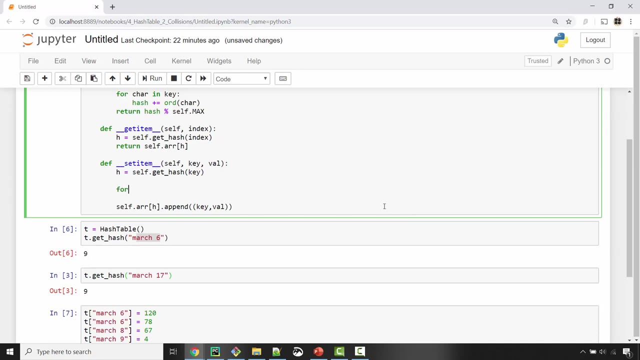 You want to update key value pair- This will be a simple scenario- But that you will do it only if the key does not exist in that link list. Hence you want to first find out if key exists or not. All right, So you will say for index element in: 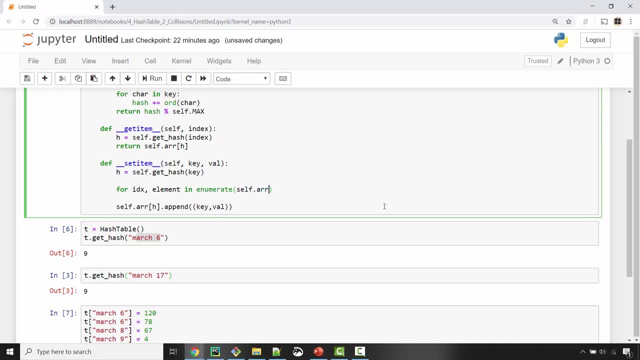 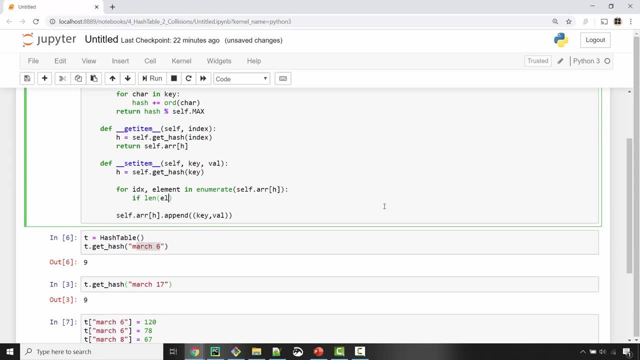 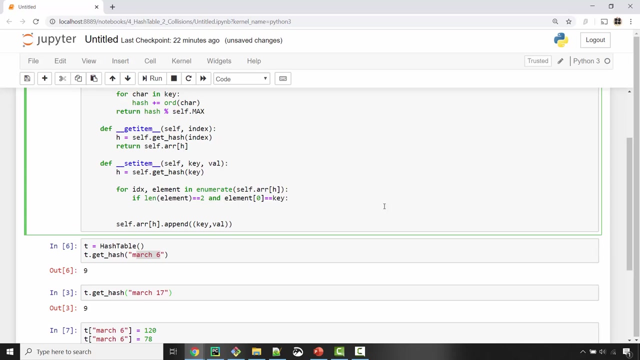 So enumerate is a function you use to iterate through the elements in your array, And if the length of element is equal to two And element zero is equal to key, which means for this key I already have an element, So that element you just change a value. 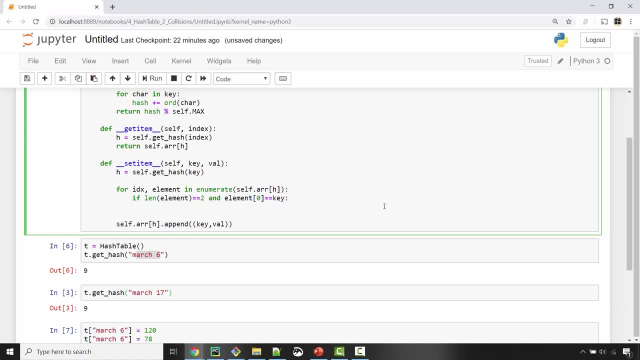 So in that same element you will change a value. But since we are inserting a tuple, our tuples are immutable. So I cannot just say element one is equal to value. you know, instead of tuple. If you had used Another array it might have worked. 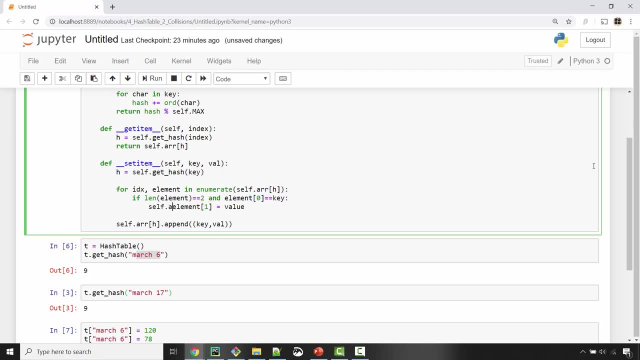 So I'm just going to insert a new tuple, basically at the same location. So my location is first of all this, And in that, on that particular index, I will store this key value location. I hope it makes sense. If this is a little complex, I would suggest you debug this in PyCharm. 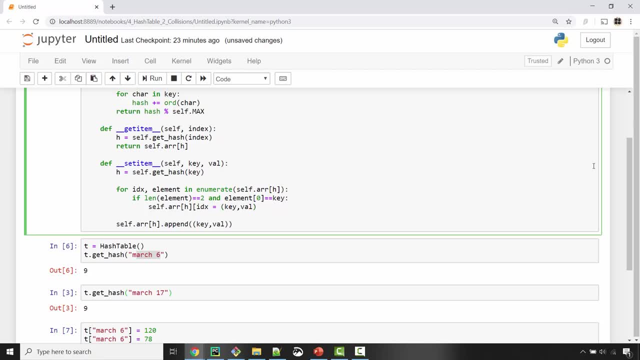 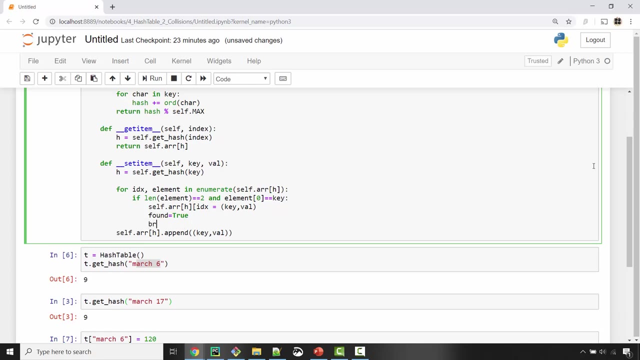 And when you step through the code, you will get an exit ID Of what I'm trying to do here, And this is found equal to true. So that happens: The found thing becomes true and you break out of the loop. Okay, so let me break out of the loop. 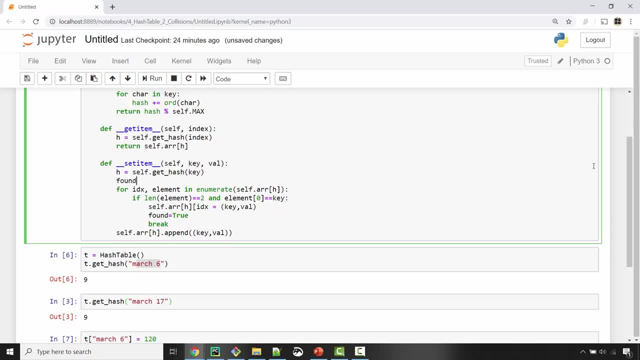 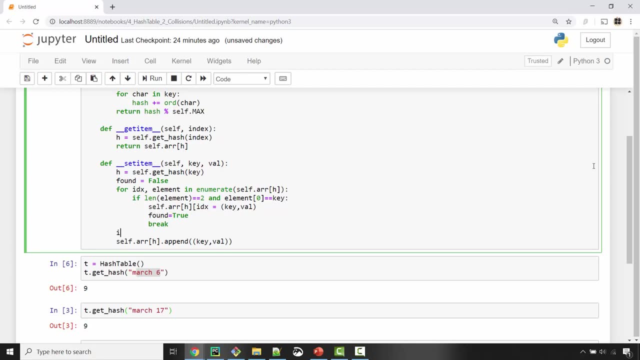 So found element is false Initially, Okay, and then you do this thing If your element is true. If your element is false, was not found, which means i did not have this key in my hash table. that's why i'm inserting it fresh. 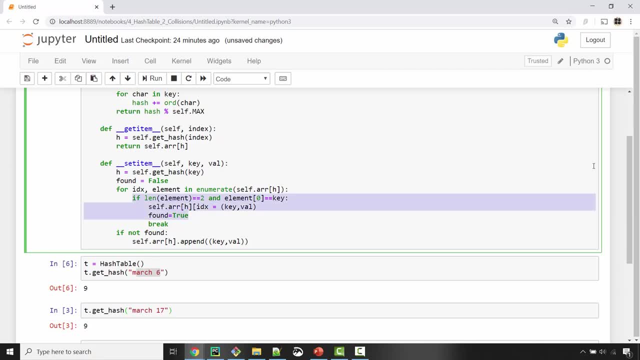 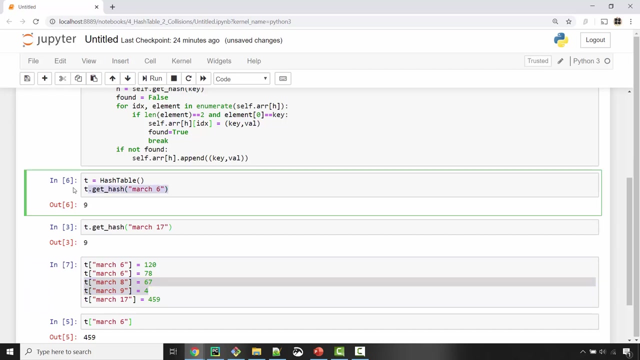 but this scenario is to handle if the key already existed. and if it already exists, you are just modifying that key value pair. okay, so i hope that makes sense. uh, let me just run it. so i did ctrl enter and it executed. now i'm gonna do: let's say this, okay, so let me remove this two things. 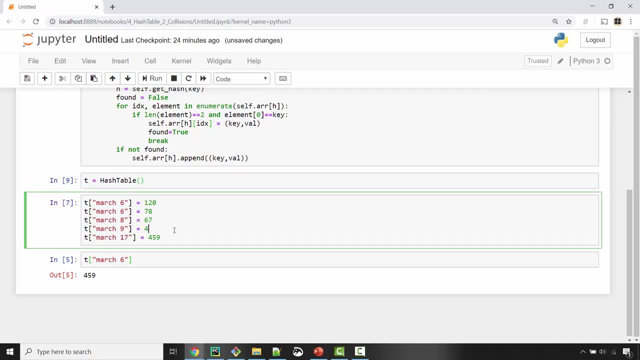 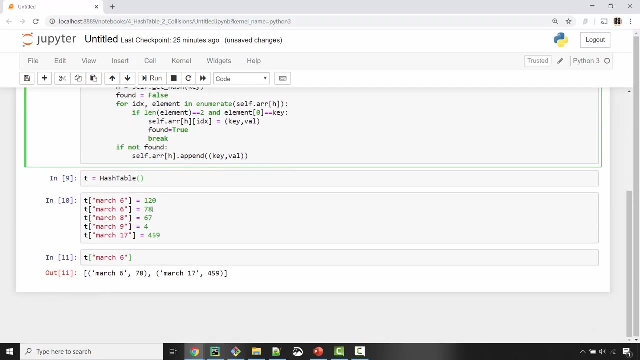 so that one is gone. so here i created hash table object and here i'm inserting couple of values and in the previous implementation, mas six was showing 459. so let's see, so here this is working correct. I mean, I don't have get item implemented, that's why it showed like this, but you can see that at that. 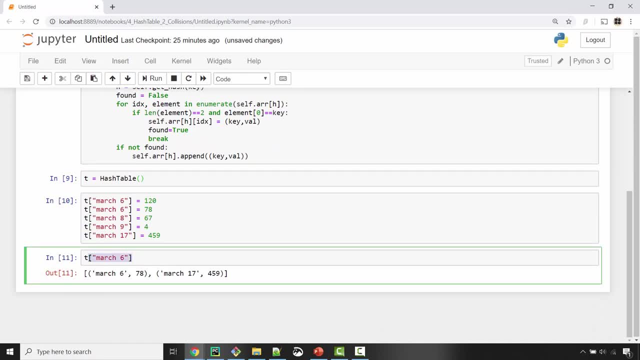 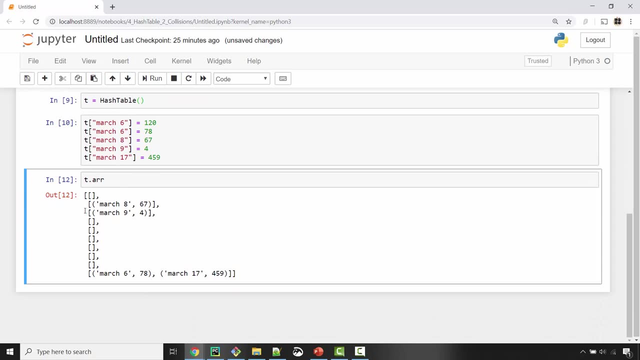 location. now it is storing a linked list. if you want to get a better idea, you can just print this array. see: in this array now every element is a list and that list has a key value pair. so March 6 and 17 gave a hash of index 9. so I am at. 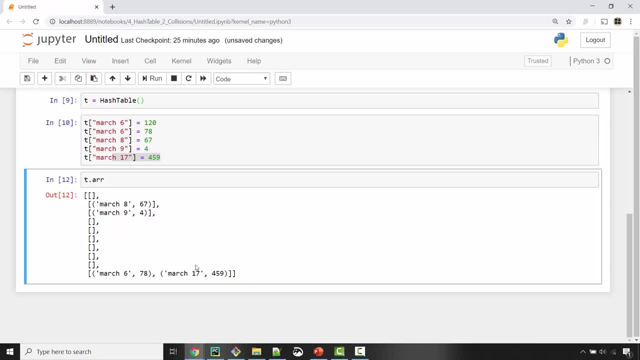 index 9, and here I have stored all these elements. so now I can modify my get function in the get function. what I'll do is I first get the index and then I iterate through all the values in that index and I try to return the value that matches this particular key. so let's modify our get item function. 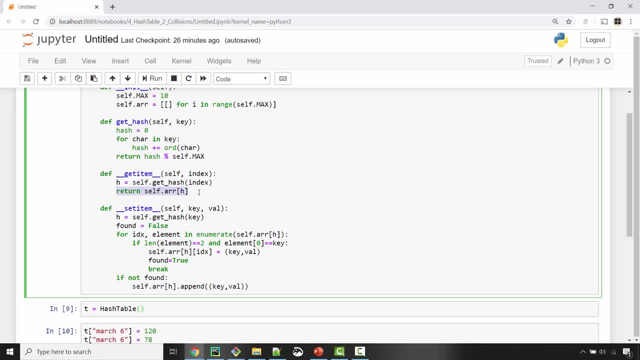 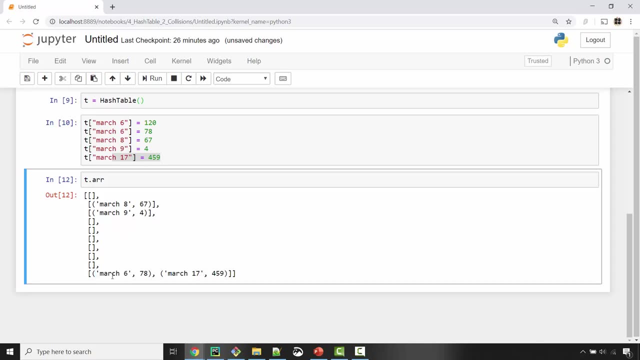 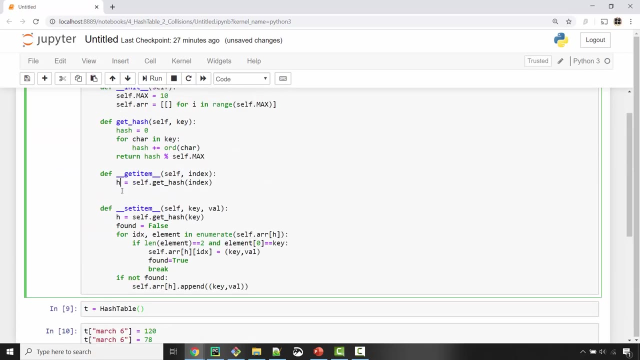 okay, okay, this part remains the same. you always want to get the hash. so, for example, just visualize you are calling get item for March 6 or March 17. in that case this hash H will return value 9. okay, and when you have 9 now, when I do self dot array, 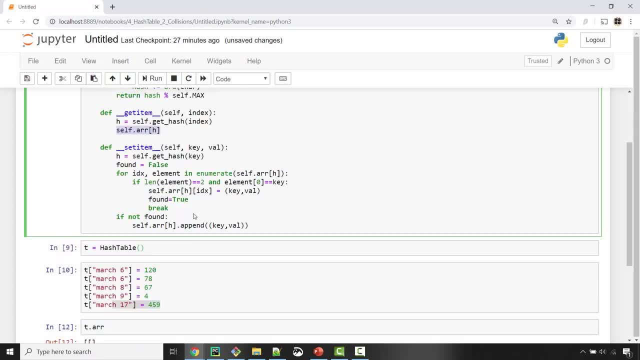 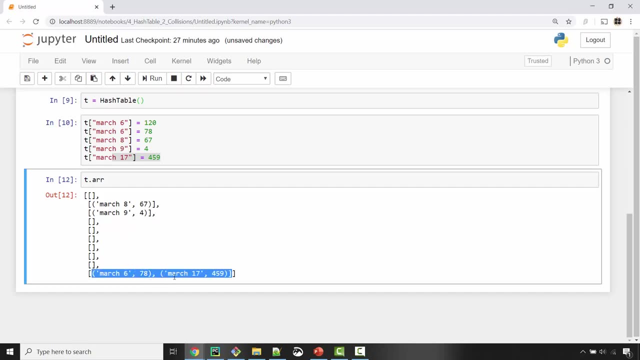 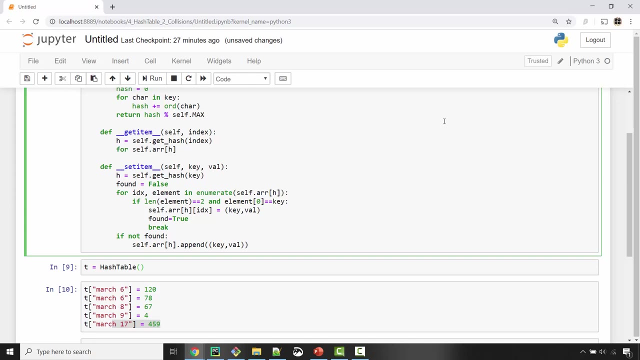 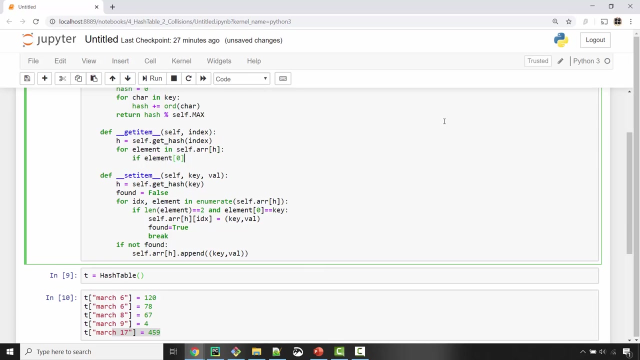 H. okay, this particular thing returns me this list, this whole list. it will return. so now I want to go through each of these elements in the list by running a for loop and find out the appropriate value. so I will say, let me just change this to key. so for that key, which is March six seven, 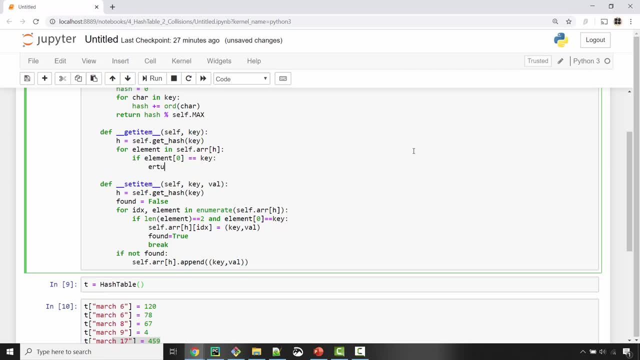 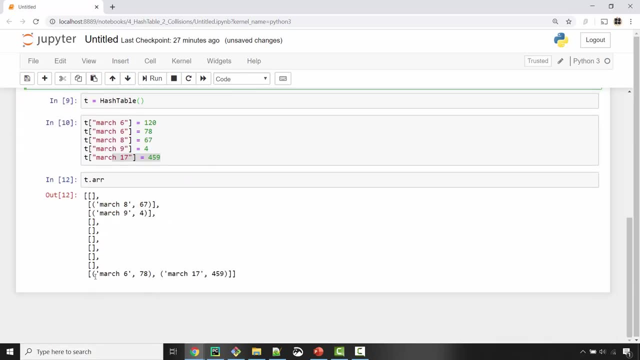 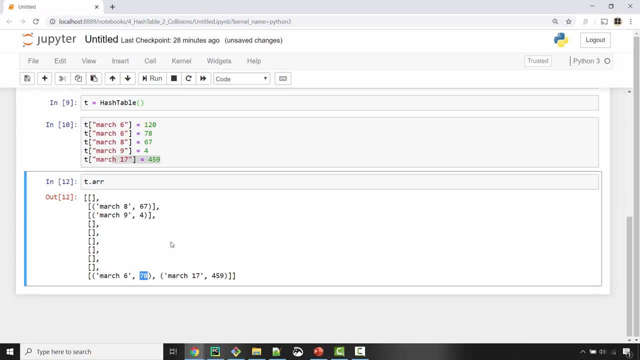 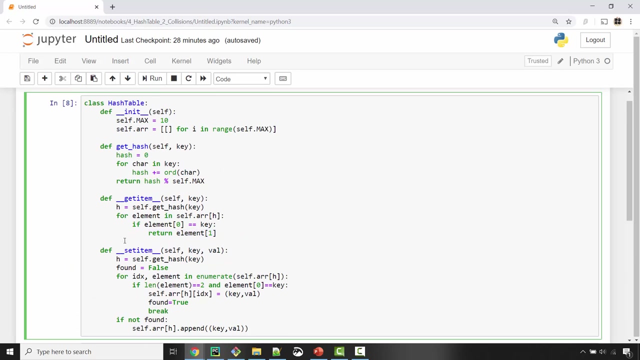 whatever. if that matches, you return element of one, see element zero. is this key which we are matching? if it matches, return the second part, which is the value itself. alright, so this looks good. if it cannot find the air value, then it will return none. so when you don't return anything in 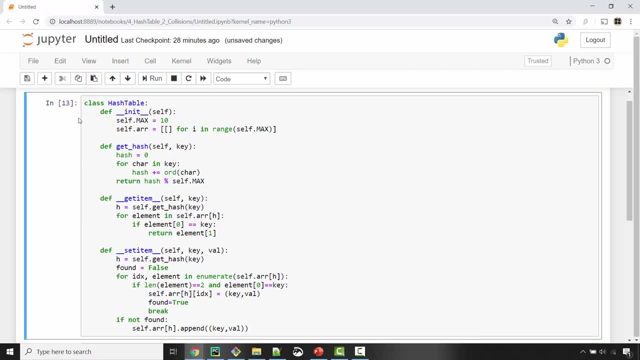 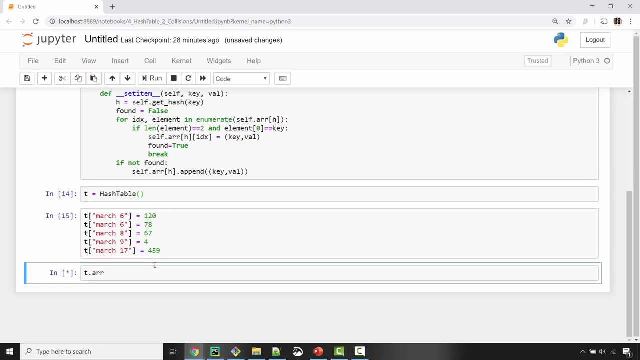 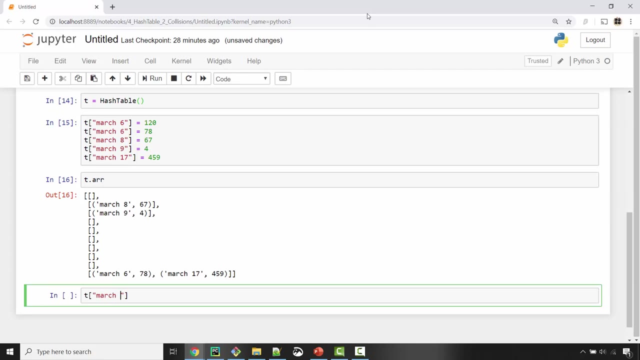 Python by default, it returns none. so control enter, this thing is executed. control enter again. control enter, control enter. so I have these values. now let me do this: March 17 or my six. see my six is coming 78, which is the correct value, and when you do my 17 it will be 459. so 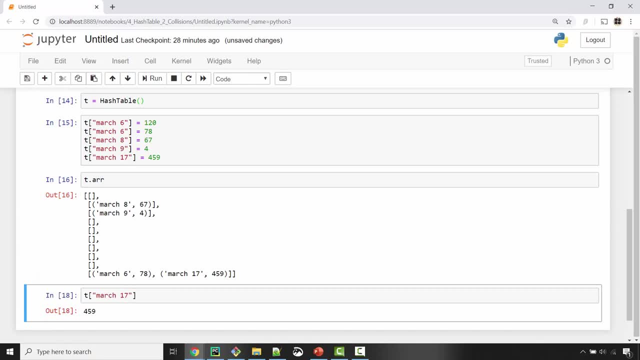 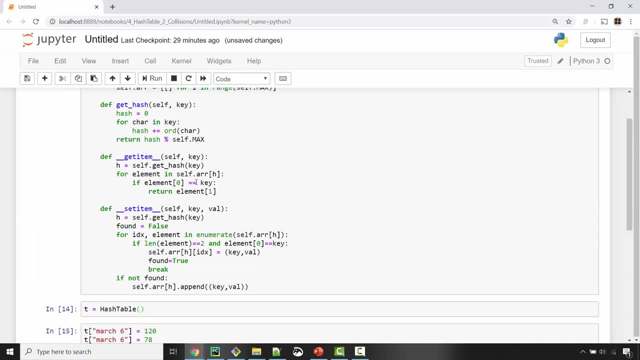 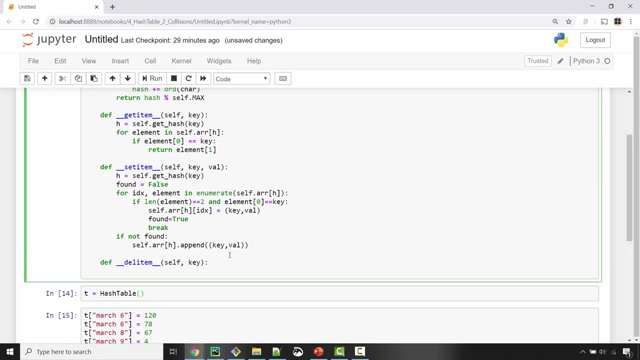 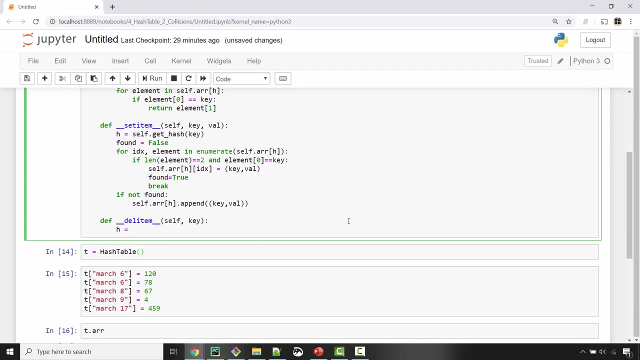 now this is working. this fix the problem that we had with the previous implementation of hash table. let's also implement our delete item function. so delete item can be implemented by overriding this method. these are all the python standard operators. okay, so delete item whenever you want to delete a key. as usual, first you will get. 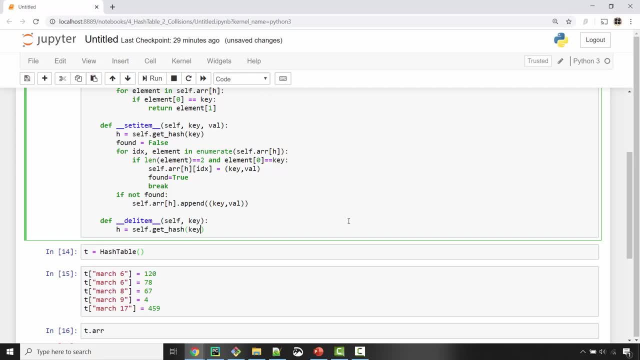 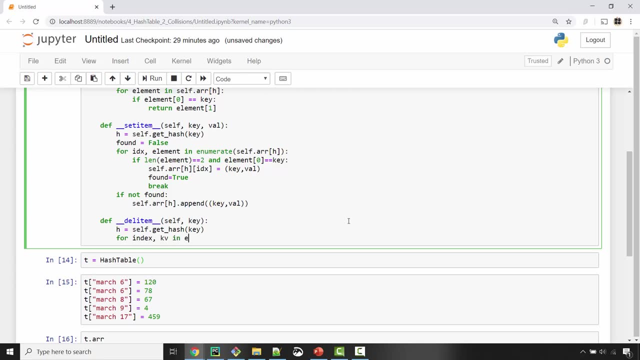 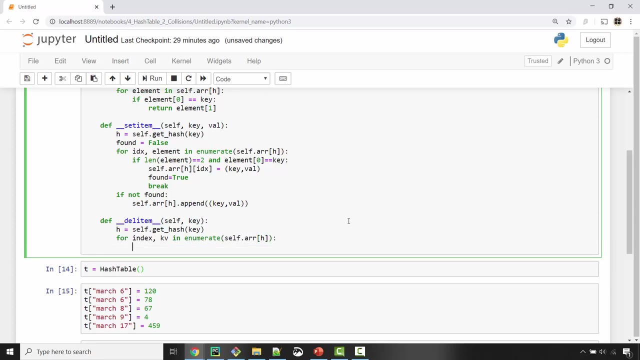 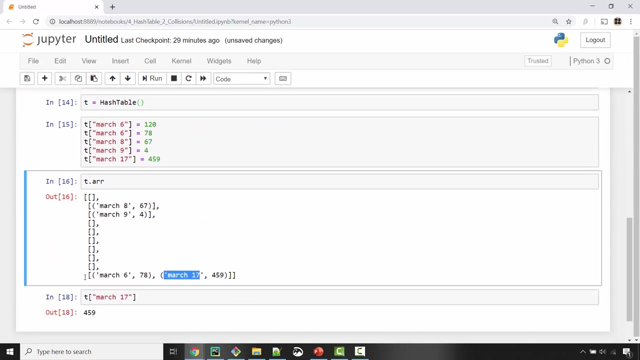 uh, self dot get hash for a key and then for index key value in enumerate- enumerate what self dot? array of H, because when you want to delete something, let's say you want to delete March 17.. you first locate the index, which is number nine, so then you get this list. so this list is this: 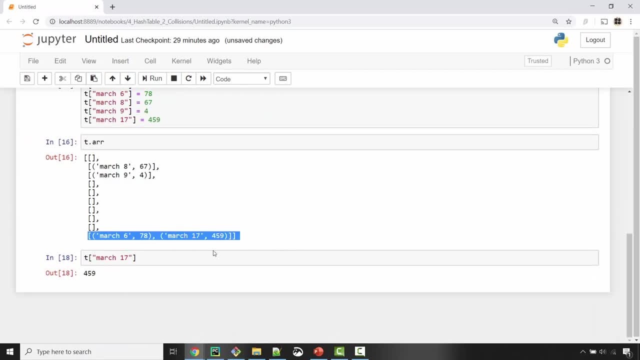 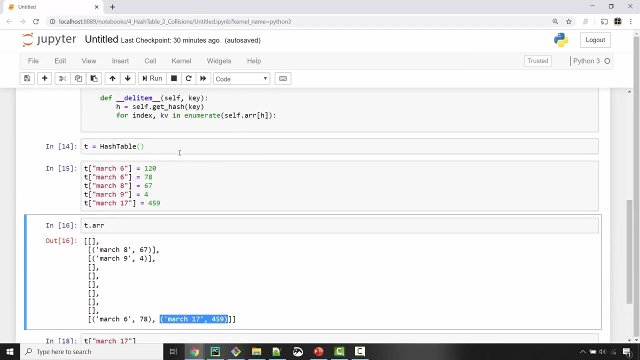 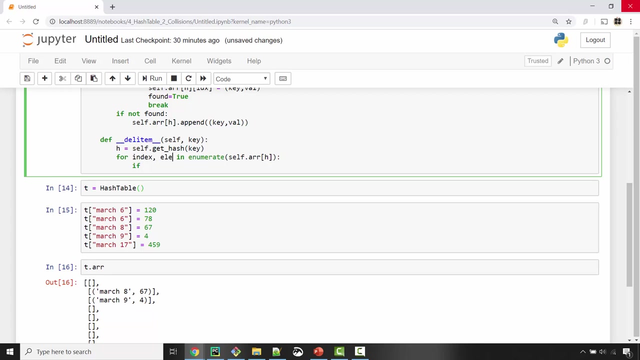 particular thing. this is that list. now you go through each of these elements in the list. so i'm iterating this loop, you can see that, and whenever you find a particular element- let's say, i find mars 17- that is something that you want to delete. so here, if instead of kv i will just use element, okay if 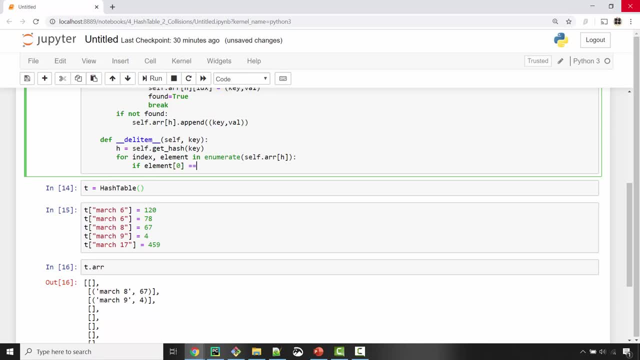 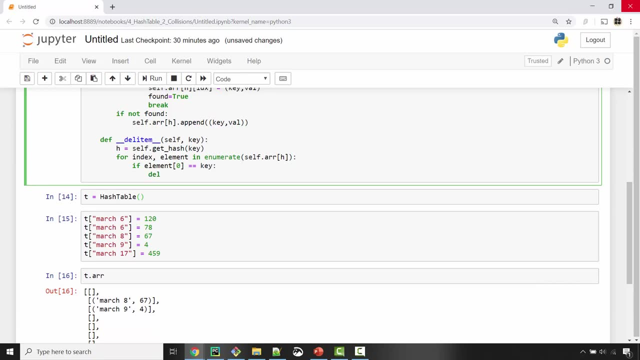 element of zero, because zero always have a key is equal to key. then we found the right element to delete and here you will say: delete self dot array h. okay, and at that edge i want to delete this particular index. so this h, let's say, if you're trying to delete march 17, this h will be number 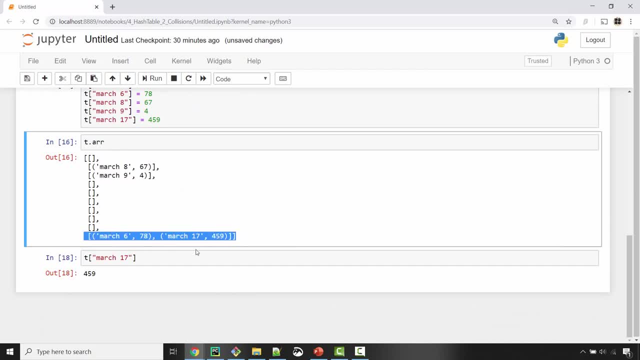 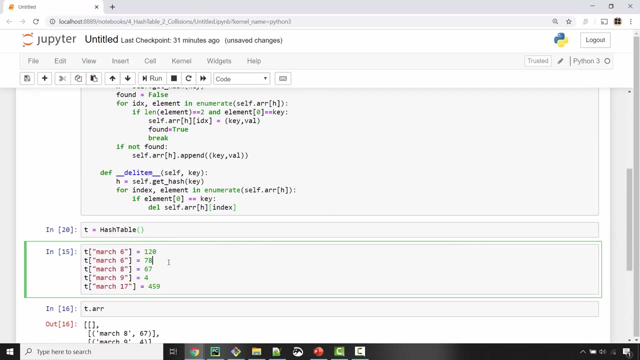 nine. okay, so number nine is this you, in that we have another list and the index to delete in that list is one, because this is zero. this is one, so one we want to delist, so that index is one. okay, ctrl enter. so this executes this ctrl. 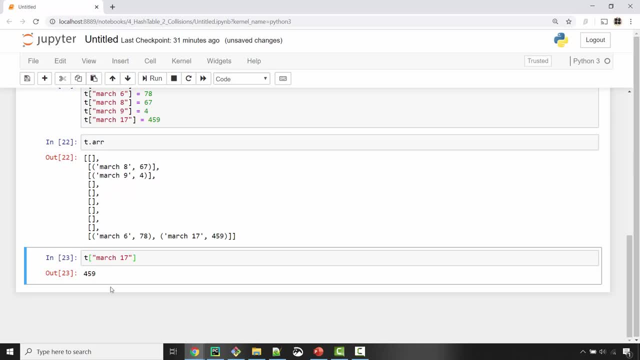 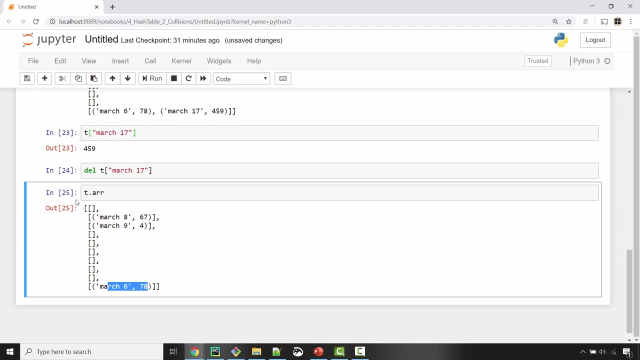 enter- ctrl enter. so i'm executing all of this, and now let's say delete. i want to delete march 17. okay, it executes. okay, it executes fine, without any complaints. but let's see if it works really. voila, now this is working. see march 6, march 17. you can also delete march 6 and see what happens. so march 6 here. ctrl enter. 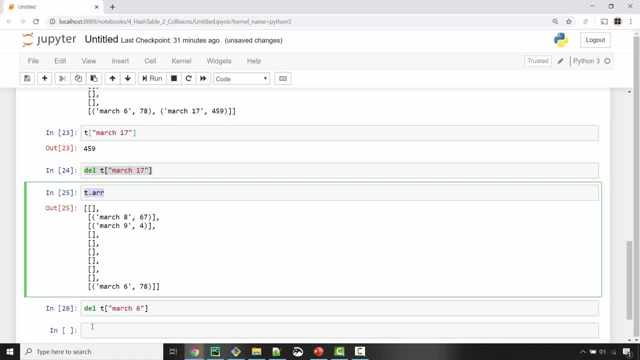 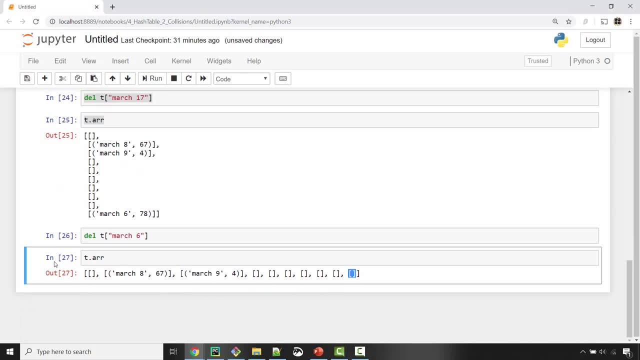 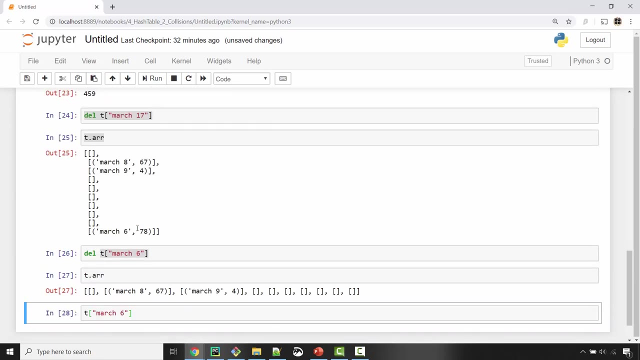 and then t dot array. t dot array- see, march 6 is also gone. that was the last element you had. now, when you try to retrieve the value of march 6, of course it's gonna return none. but you have other elements, such as march 9, for example, whose value is 4. so when you do march 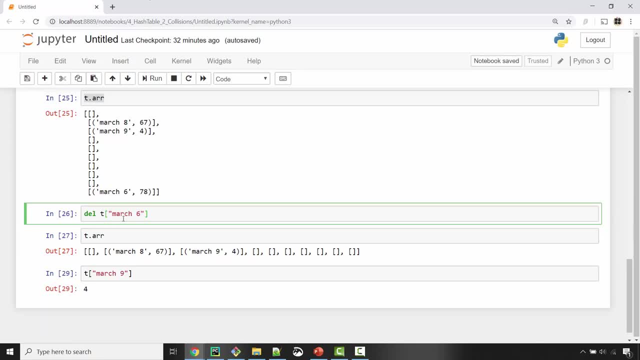 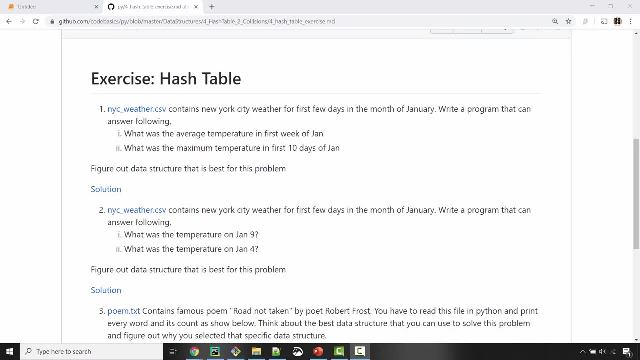 9, you get value 4 back. so this hash table seems to be working okay. now comes the most interesting part of these tutorials, which is an exercise. without doing this exercise, it's all useless guys, believe me. so you have to work on these exercises. solution links: but you will click on solution link only after you have tried it yourself. all right, so 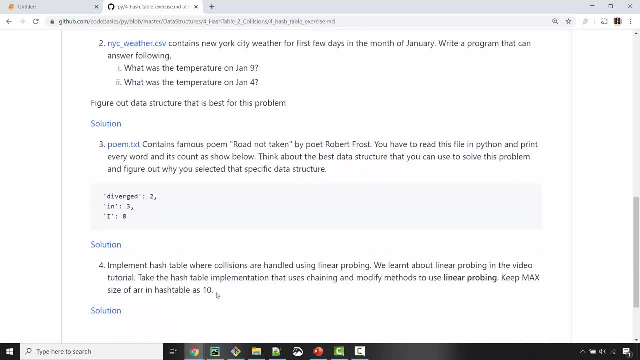 i have, uh, four different exercises. the fourth exercise is little complex, uh, where i am asking you to implement a linear probing in your hash table. but if you have already watched this particular tutorial on how to implement using chaining, i think you can get some insights from that. so just take that same class and modify it, and there are some other exercises, so read. 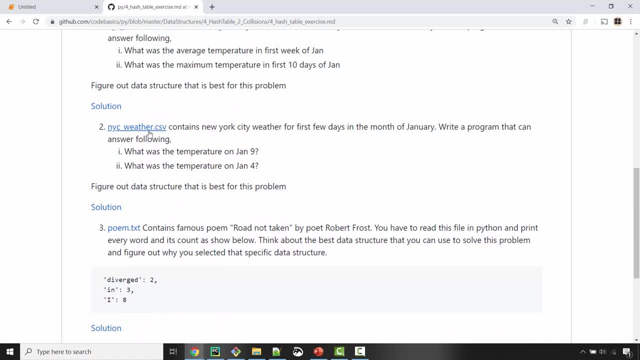 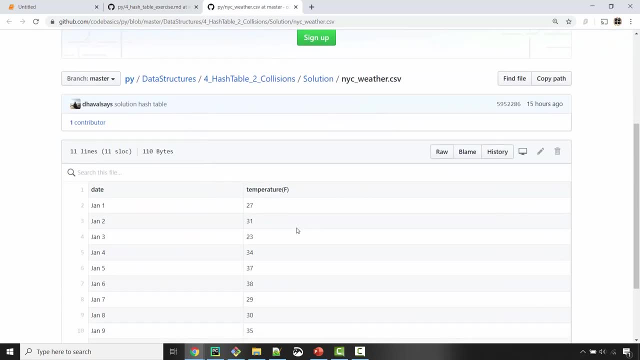 through the description and try to solve, uh, these problems. i'm also providing csv files, for example, here now, many times people ask me that: okay, how do i download this csv file? so, to download my entire repository, what you should do is you should go to the root, which is py. okay, so go here and 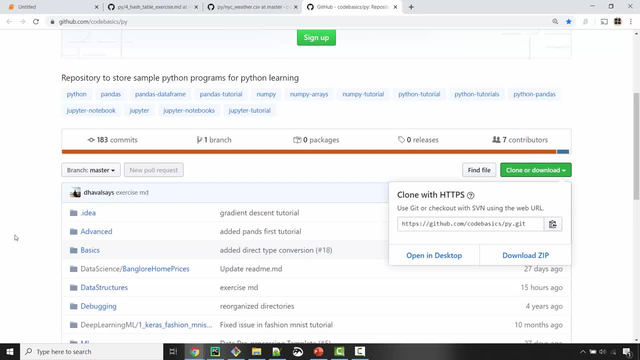 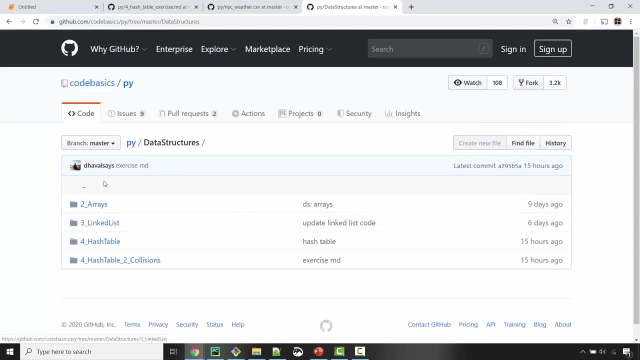 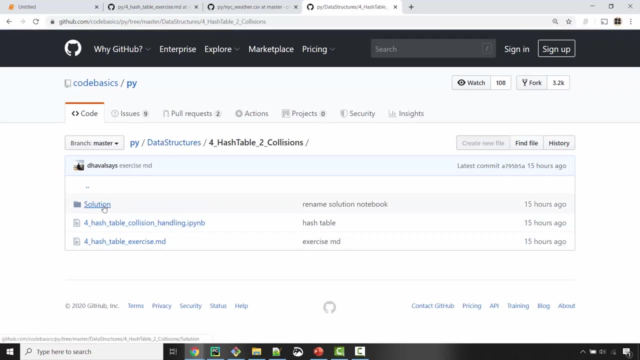 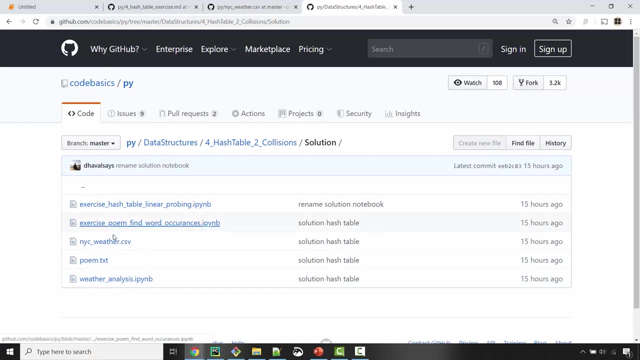 when you say clone or download, this way you can download the entire repository with all my tutorials and in data structure. so if you go inside data structure, see i have all these different tutorials and hash table collisions. when you go here in the solution, i have this csv file, poemtxt, etc. so when you clone the entire repository, 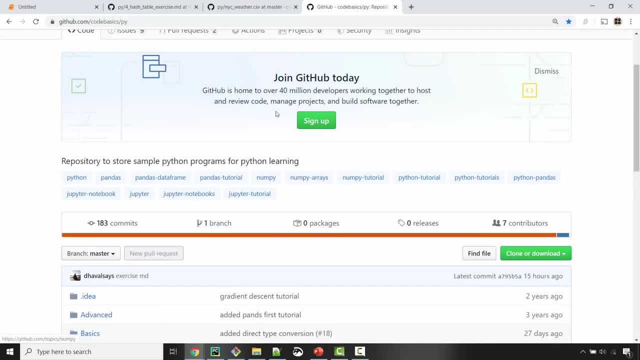 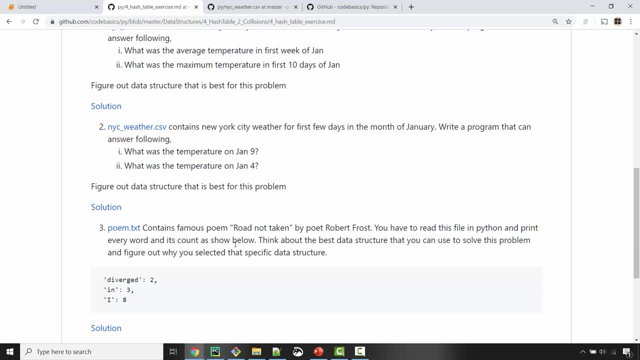 by going to pi, clicking on this green button, you will get those files. okay, so get those files, work on those exercises and post your solutions in a video comment below. you can also match your solution with my solution by clicking on this link, but first try it out yourself. so thank. 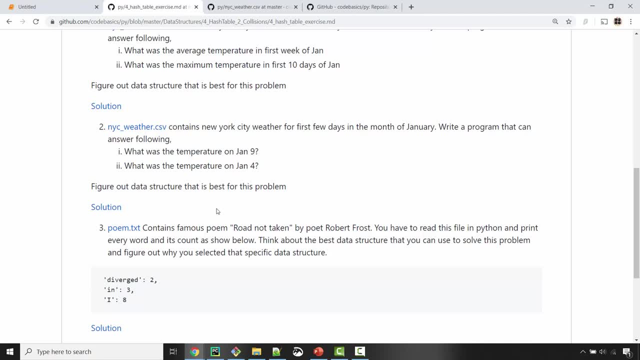 you for watching. i hope the this two-part video series on hashmap has clarified your doubts. remember, data structures is a hot topic when it comes to programming interviews or data science data analyst interviews, so having in-depth understanding of data structure is very, very important. hence, it's very much needed that. 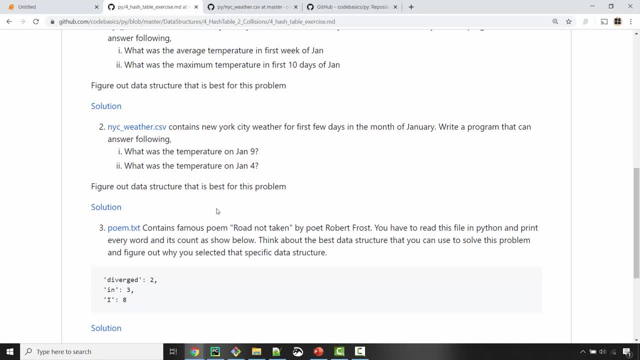 you watch this whole data structure tutorial series. you work on these exercises. you get an idea on the big o analysis between different data structures. link for the exercise, this link and the code that i went through. those links are provided in video description. so always check video description for any of my videos. i provide ton of useful videos and use them in this series. thank you and i hope this video was useful to you and i'll see you in the next video. bye, bye, bye, bye. information there.